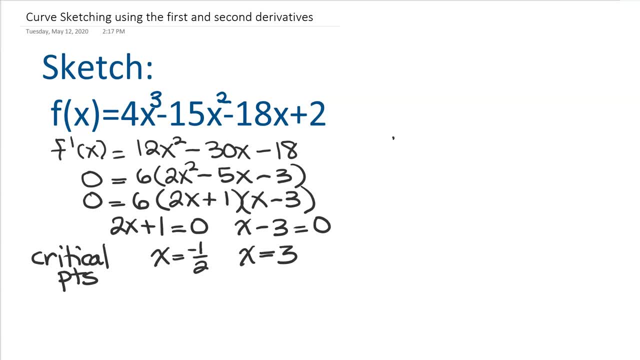 I'm going to move on to the second derivative to do this, So I'm going to take my second derivative here which, going off my first derivative using this, my second derivative is going to be a 24.. X minus 30, I'm going to set this equal to 0 while I have it, because this is where my possible inflection point might be. 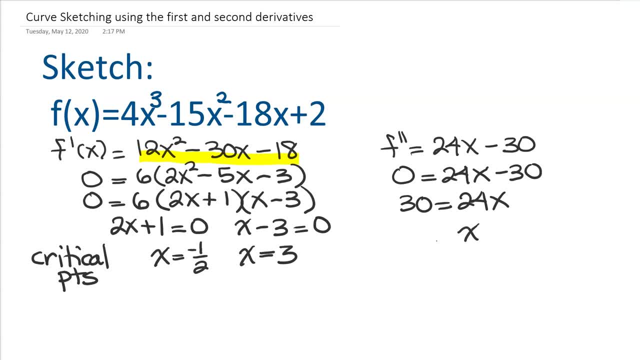 So, solving this for x, dividing both sides by 24, I end up, if I reduce it to 5 fourths. So I like to call this my PIP, my possible inflection point. I still need to do the testing to find out. 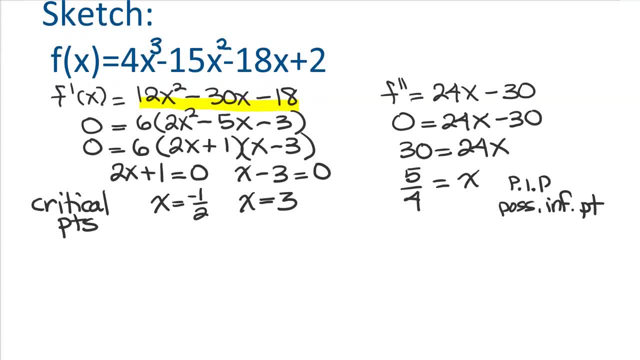 Okay, so I've got a lot of points here. Now what I'm going to do is a second derivative test, And actually I can use that to determine what all of these points are. So I'm using my second derivative. Let me put 5 fourths on here. 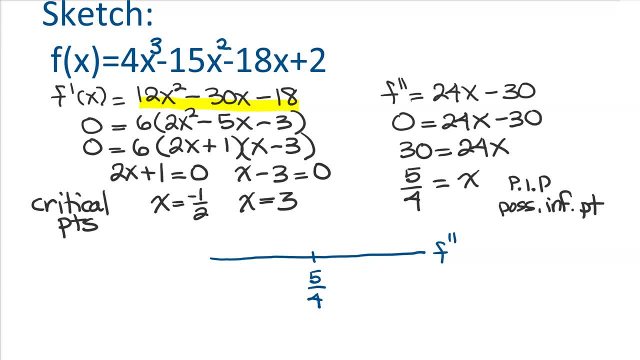 So I'm going to choose a point on each side of 5 fourths And, strategically, the points I'm going to pick are these critical points. So I'm going to pick over here. I'm going to pick x is 3.. 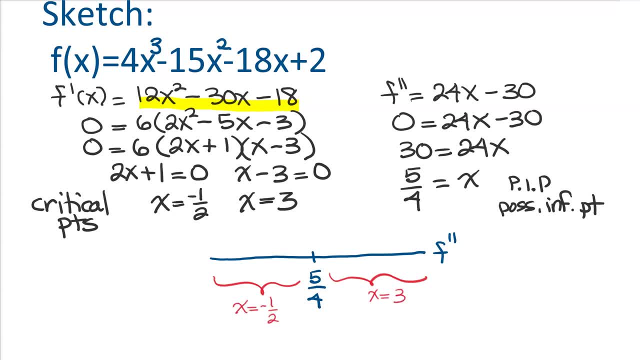 And over here I'm going to pick: x is negative a half And I'm going to plug this in These values, remember, into the second derivative, So into my 24x minus 30. So when I do that, and again you may want to pause so that you can kind of do this yourself. 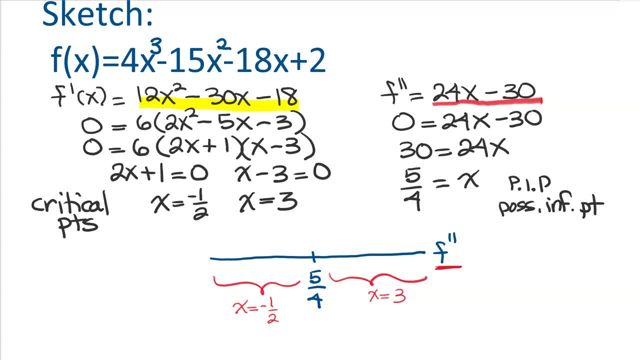 Use your calculator, plug them in. When you plug 3 into your second derivative, you end up getting a positive value. And so what that means for your second derivative: when that is positive, that means you're happy that you are concave up. 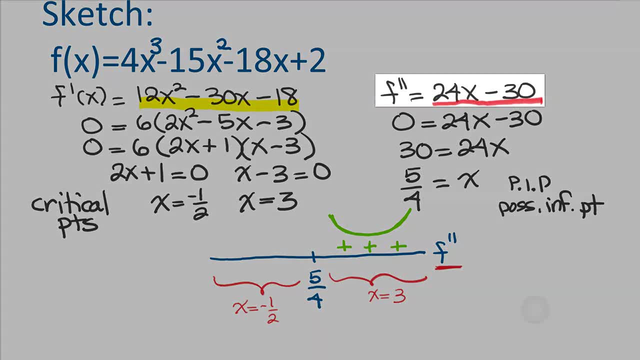 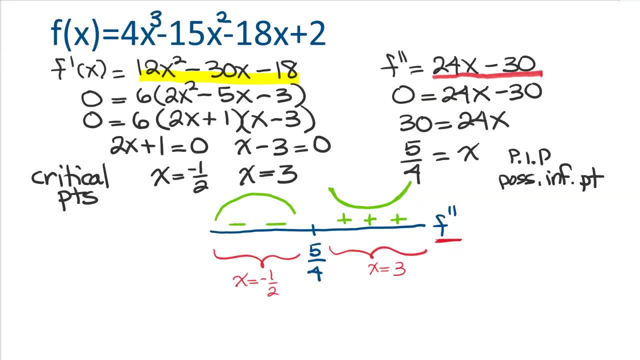 Plugging negative a half into your second derivative, you're going to get a negative value, And a negative second derivative means you are sad, you are concave down. So this gives me a lot of information, For one thing, because 5 fourths is a place where the concavity changes. this is definitely where my inflection point is. 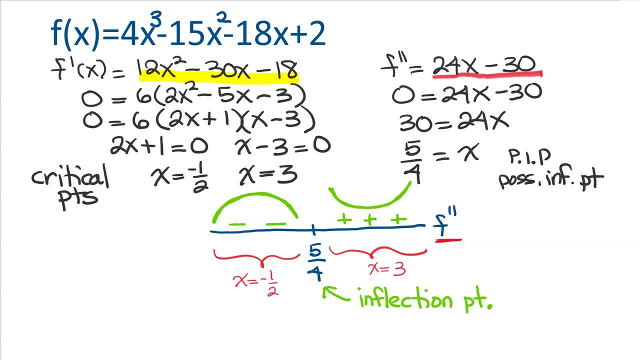 The other thing, because I chose to plug my critical points in the second derivative. then what I know is that this critical point of x is 3. Because the second derivative is positive and facing up that this guy must be a minimum. And for the same sort of thinking, this other critical point: when I put this in the second derivative and I got a negative. 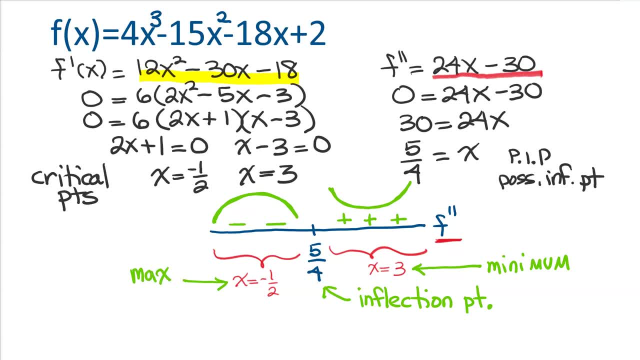 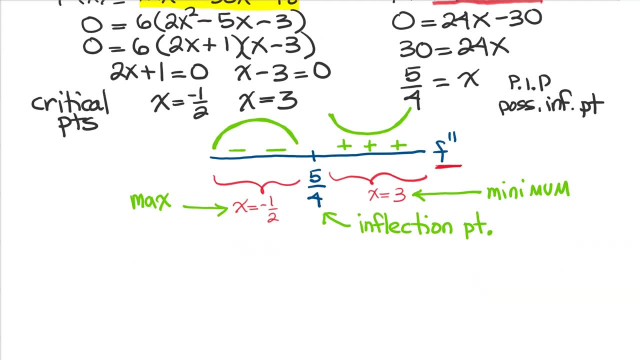 that means at this point I must have a maximum. So I've got all kinds of good information here. Now what I need to do with every one of these is to put them in the second derivative. And what I'm going to do with every one of these points is I need to plug them back into the original function. 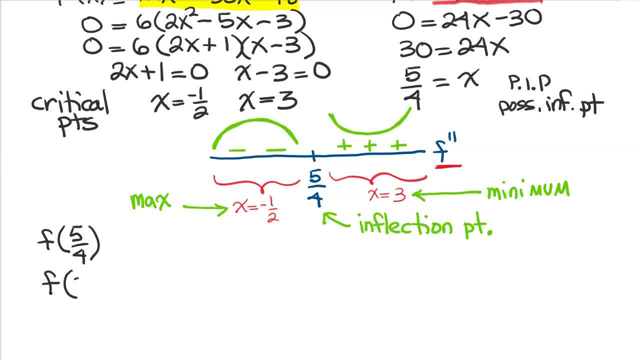 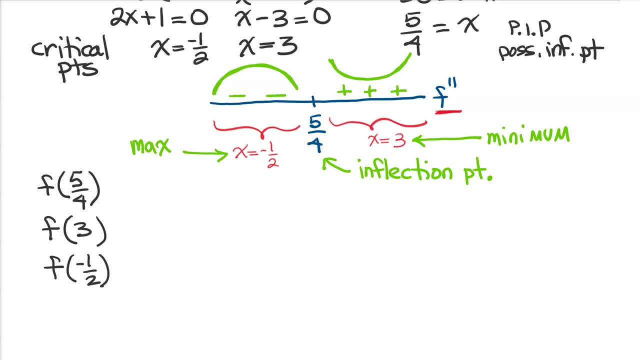 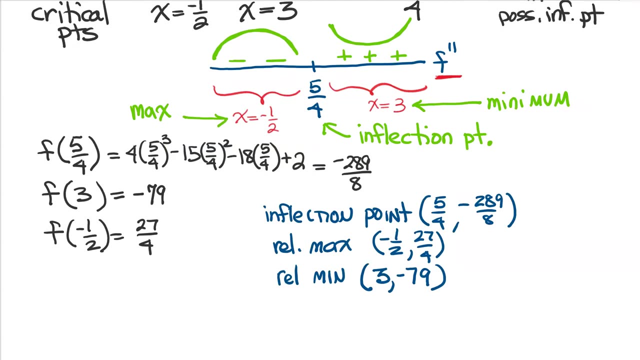 So I'm going to plug 5 fourths into the original function, I'm going to plug 3 into the original function And I'm going to plug negative a half into the original function. Okay, so here's the results, Plugging these values into my original function. 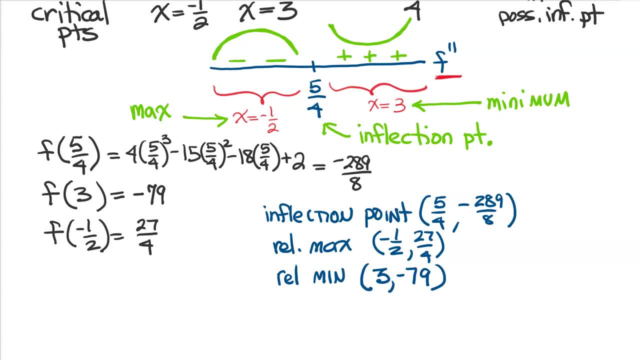 I've got these y values to go with my x values, And so I'm ready to sketch My function now. I've got a pretty wide range of y values- This negative 289 over 8, that's about negative 36, and I've got negative 79.. 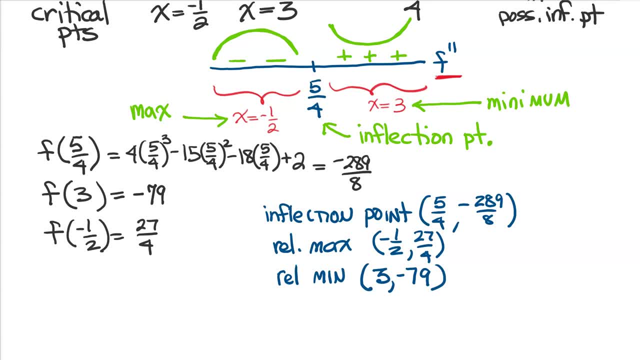 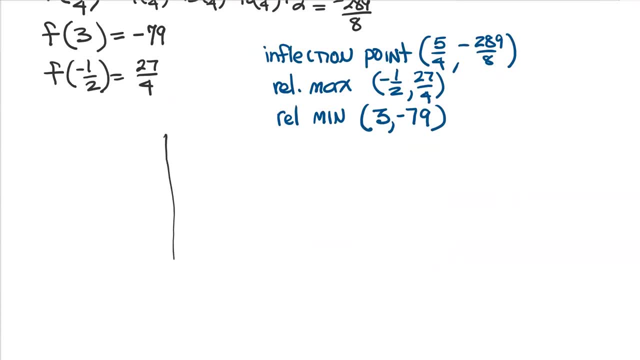 And then the highest y value I have is about 6.75.. So you know my graph is going to be quite a stretch here, So let's just do the best we can. We know that we need our y axis to go down at least as low as negative 79.. 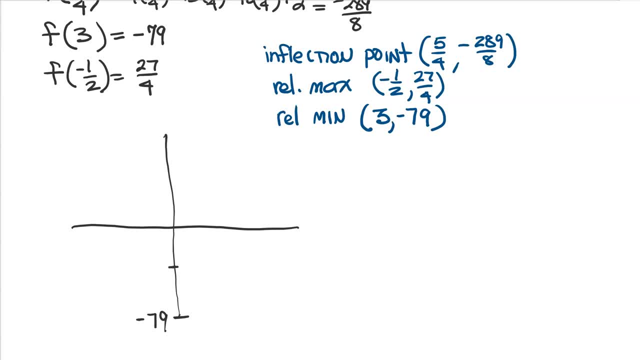 Also in there we'll have our point at about negative 36,, which is really negative- 289 over 8.. And then the highest y value we have- and again this is not to scale here- is the 27 over 4,, which is really about 6.7.. 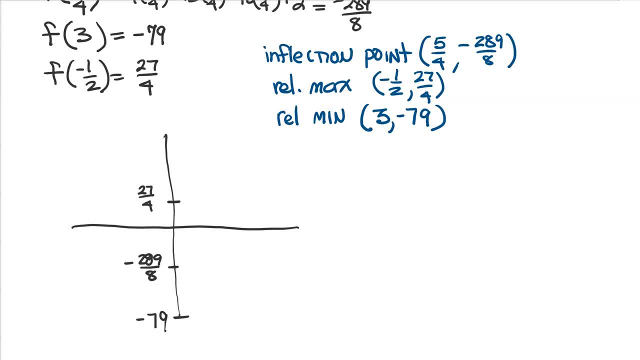 So the x values that we need to graph. we need a 5 fourths which is about 1 and a fourth. We need a 5 fourths which is about 1 and a fourth. We need a 5 fourths which is about 1 and a fourth. 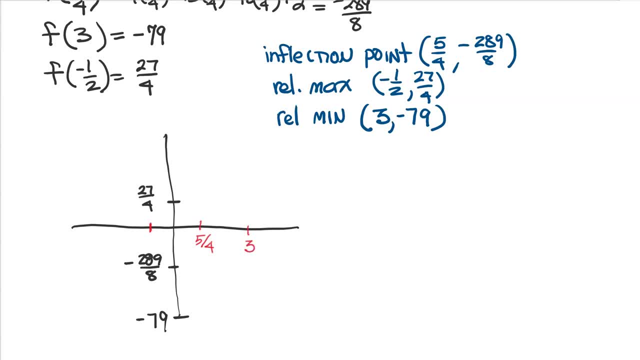 But we need to have an x value of 3 and we need an x value of negative 1 half. So I'm just going to plot these ordered pairs on here and then I've just got to connect the dots the right way. So I've got 3 and then my negative 79..